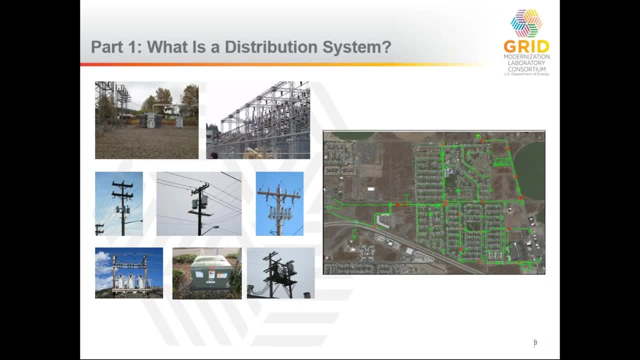 if you ask a graduate student what is an electric distribution system, they'd give you an answer that looks like the picture on the right there. That picture on the right is a one-line diagram in a distribution system planning software overlaid on Google Maps, and that's the way. 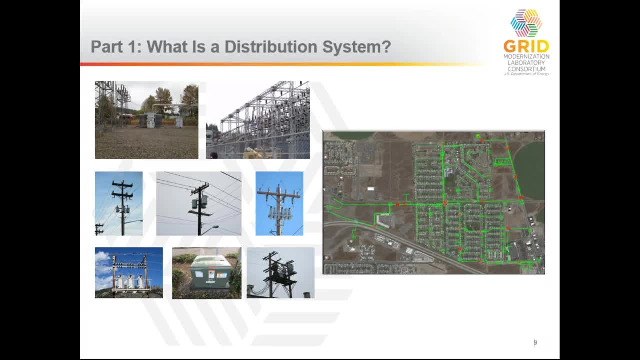 a planner would work at it, but when you're actually on the ground, you start to see the equipment that's at the left, the various pieces of equipment that exist in substations, out in the field, and these are the devices that each of them serves a critical purpose If they fail. 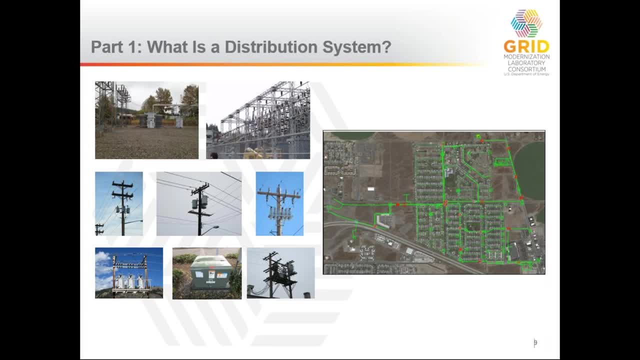 typically, that means there'll be a service interruption and there's different ways to accomplish the roles that they fill, and it's good to understand what these are and what they appear to look like. Next slide, please. So within North America, the characteristics of a modern 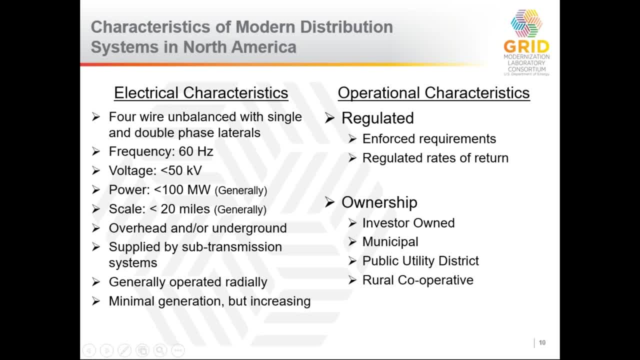 system. We use what's called a four-wire unbalanced system. What this means is that we have three conductors that provide power and a neutral line, and I'll talk about that a little bit more in detail as we go further. In North America, we use 60 hertz Voltages at the distribution level. 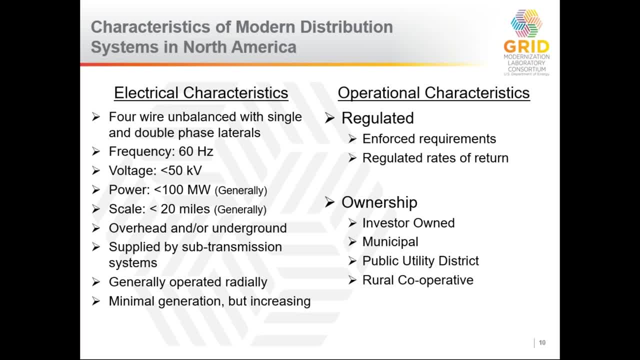 are typically less than 50,000 volts. More like 12,000 is much more common. Power levels, when you're talking distribution level equipment: less than 100 megawatts and for a distribution level: less than 100 megawatts And for a distribution level. 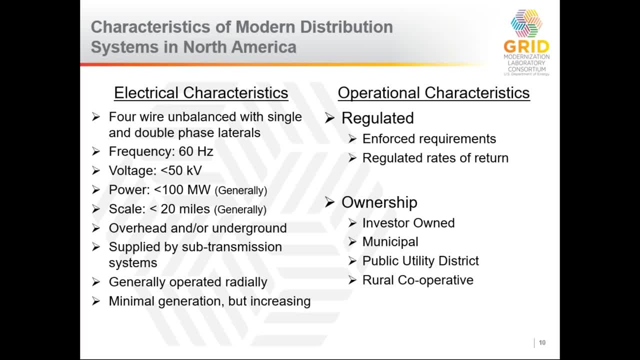 distribution circuit power only goes less than 20 miles. There are exceptions, but these are good rules of thumb. We use a combination of overhead and underground lines here in North America and for the most part power is supplied from the sub-transmission systems. These are the bulk power. 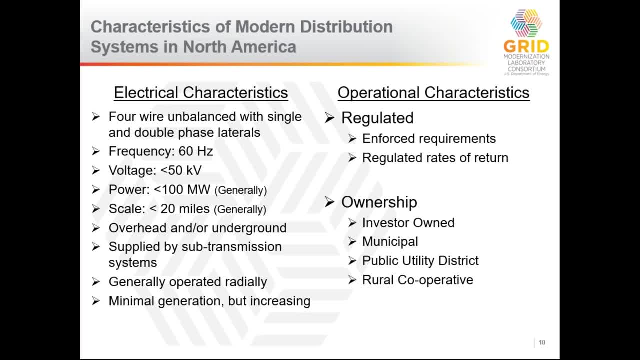 systems that bring power into the region. Distribution circuits are almost always operated radially. What this means is that there is a single path of power to flow from the substation to each house. That's a very cost-effective way to do it, but there are some reliability issues, because if you 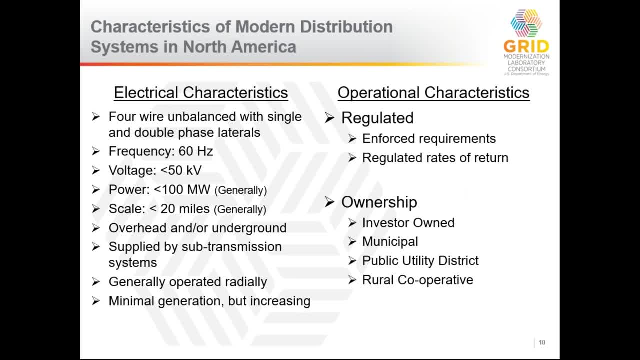 have a break in there. there's no power, But these can be rerouted manually and sometimes automatically, which I'll talk about later. At the distribution level, these systems were historically designed not to have any generation. However, this is increasing, We know, in areas such 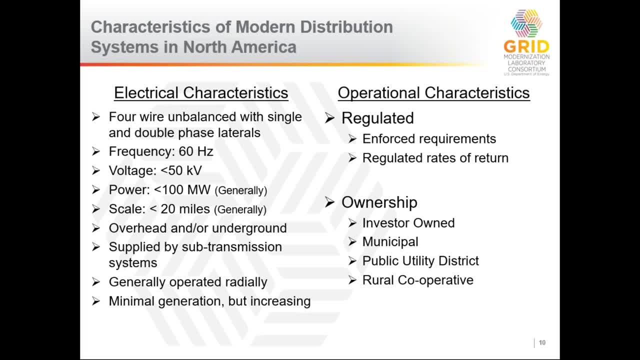 as the Carolinas, Hawaii, California and others. we're seeing a lot of solar generation go on and that's fundamentally changing the characteristics. When you look at the operational characteristics, utilities in North America tend to be regulated where you have enforced. 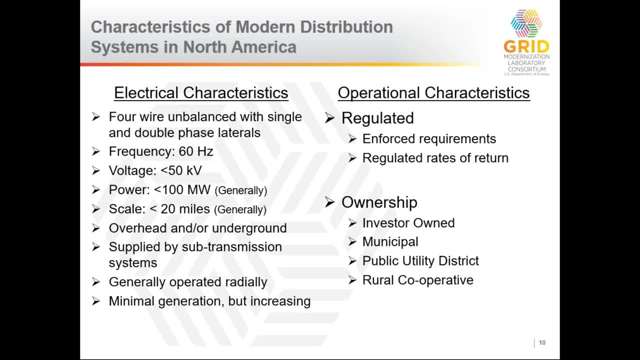 requirements, regulated rates of return, and so it's not the Wild West. in a business sense, Things are very well thought out, and what that means is that the technical decisions are almost always driven by the regulatory environment, And we have different ownership models for public utilities or distribution utilities. in North America, The investor-owned 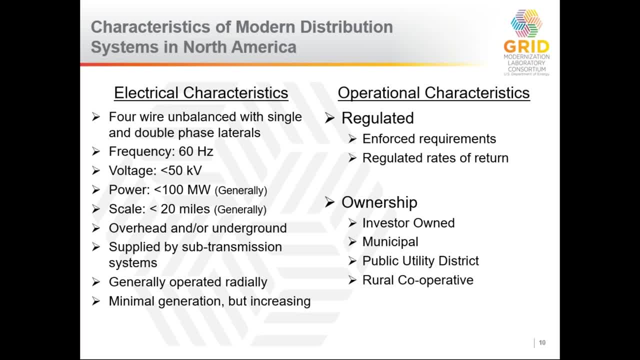 these are ones that they are publicly traded. owned stock may exist. Municipal utilities: they're run by local cities. Typically, their service territories can't extend outside that area. The rural co-ops: they exist in every state of the union and cover something on the order of. 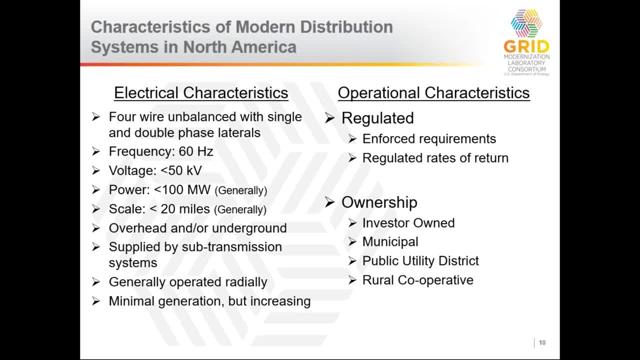 70% of the landmass. Historically these serve just rural areas, but the name's misleading because in some cases they supply very urbanized areas. And then in some areas, such as Washington, Oregon, we have public utilities. they're run by local cities, but the name's misleading because in some 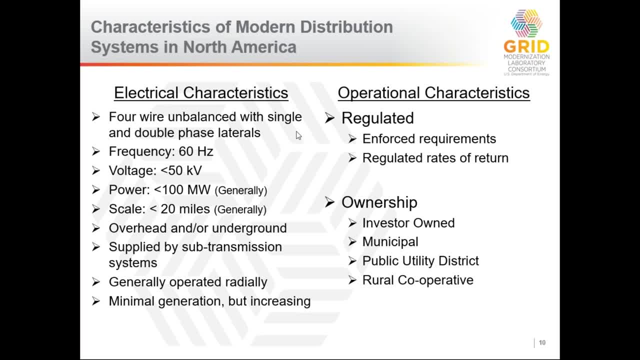 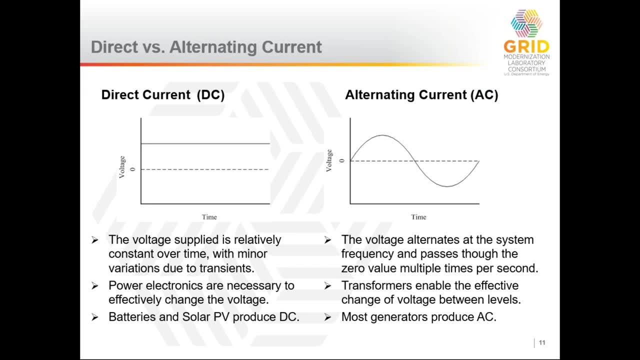 public utility districts. Next slide, please. So an important part of the underlying operation is the type of current that we use in these systems. Many people are familiar with direct current, which is what you would get out of a battery, Basically the current that flows out. 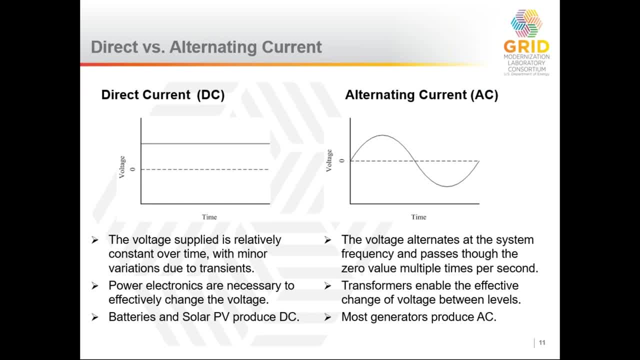 or I should say the voltage that comes out of it over time is constant, more or less. This is what a lot of power electronics run on. This is what you'll see in your car battery. However, they don't interface very well with DC systems And in this case you require power electronic. 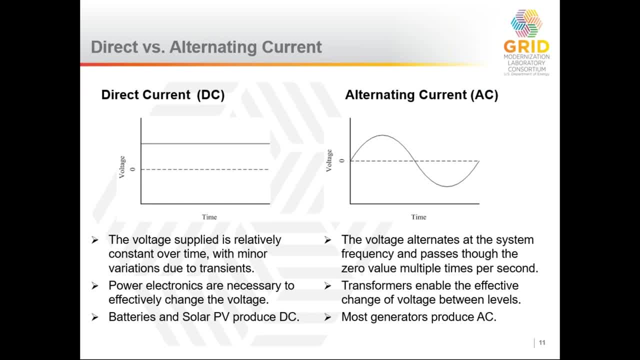 converters to convert it to an alternating current, which we see on the right. In alternating current, the voltage 60 times a second will pass through zero in a sinusoidal form. The reason for this is that with alternating current, you can effectively use transformers. 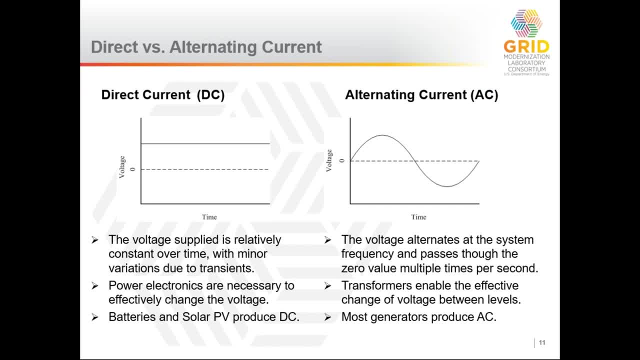 to change the voltage, And this is what allows us to move power over long distances, And it's why AC originally won out over DC in the original Tesla Edison battle. With alternating current, you can generate power at around 20 to 30,000 volts. However, you can't move it very far. 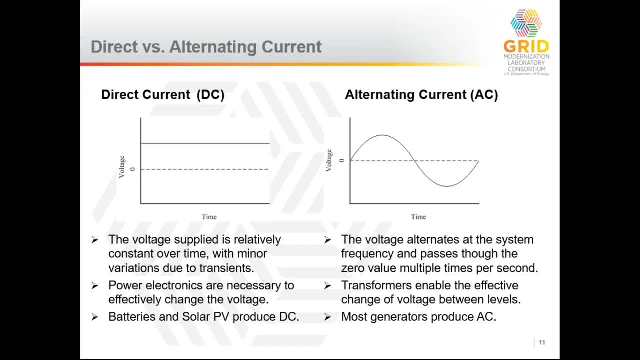 at that voltage. So it's generated, that voltage stepped up to 230, 500 in the Northeast up to 765,000 volts. It can be transmitted long distances and then stepped down to distribution level voltages. That ability to cost-effectively generate power over long distances is what we're. 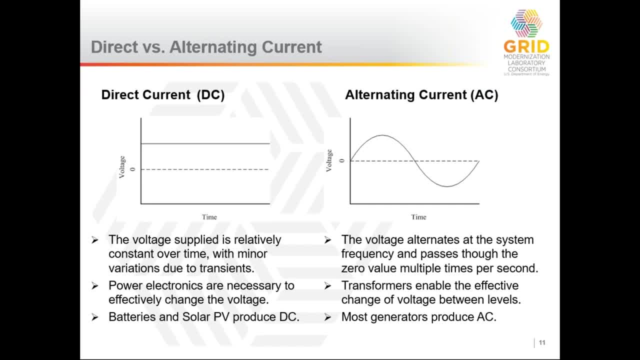 going to see in the future. So alternating current is going to effectively change the voltage is what makes alternating current such a common use today. With that said, power electronics are making the ability to transfer voltage more and more cost-effective, So we'll see more direct current in the future. However, utilities will be primarily using 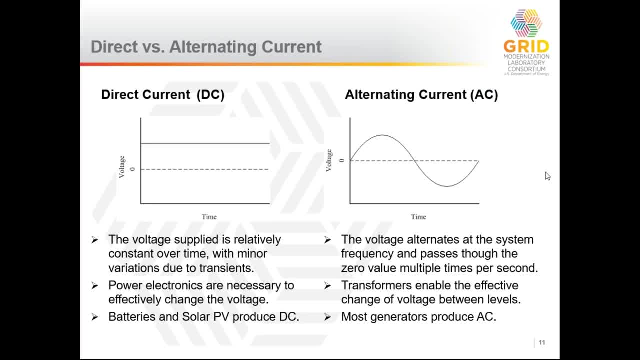 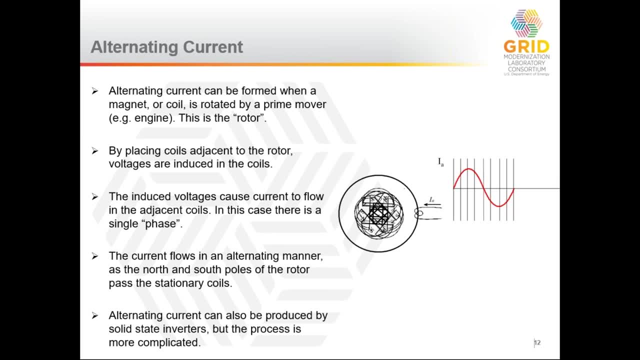 alternating current for the foreseeable future. Next slide, please. Alternating current is typically produced by taking a coil, whether or it should be called a coil, let's say a magnet or an energized coil. You connect it to a prime mover, whether it be a steam. 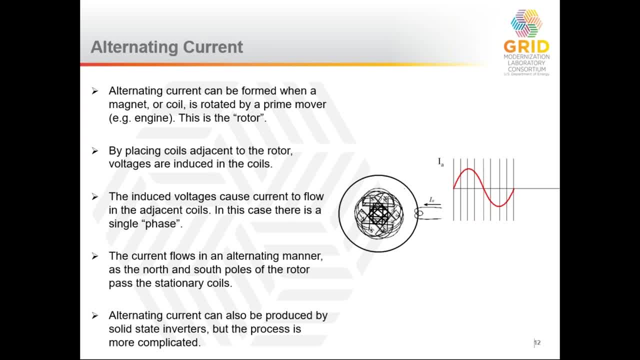 turbine, a gas engine, a hydroelectric turbine, and this rotates it around. This becomes your rotor. If you put coils next to that, you'll get induced voltage in it in a sinusoidal form And this is what produces a simple alternating voltage waveform. Folks may have done this in 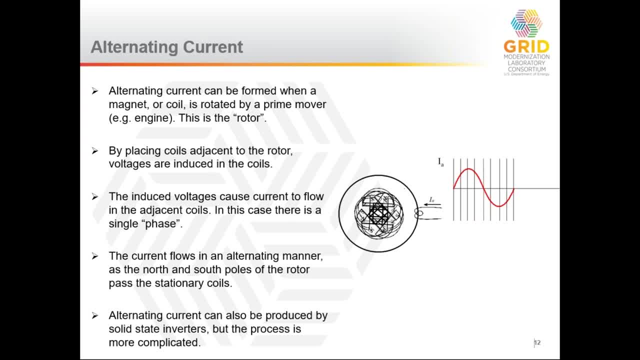 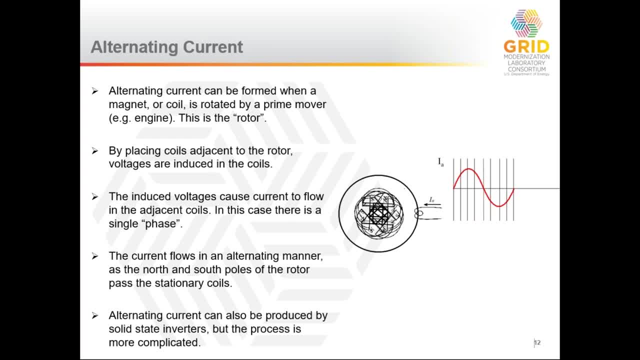 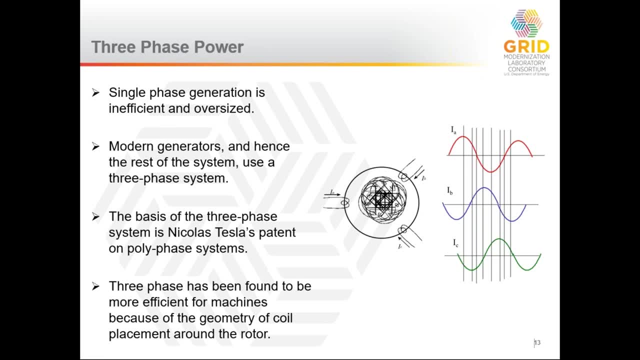 But it's how, historically, we have produced the alternating current that is used in all of these systems. Next slide, please. Now, making just a single phase of power doesn't make. it's not very efficient from the geometry of machines. So what we've ended up doing is using 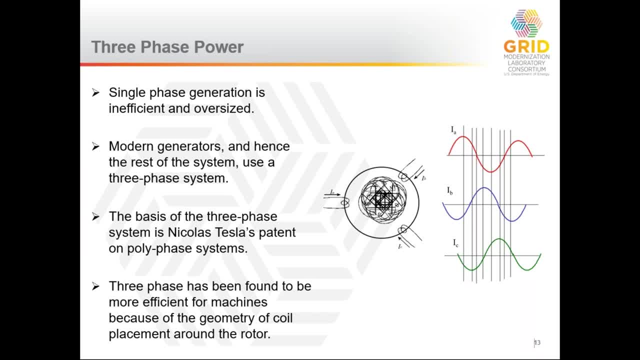 a three-phase system. Pretty much every major generating station in North America will use three-phase generators. Smaller generators that you would use, say, on camping or an emergency, maybe a single phase, But that's because that's the connection of the house For our large central power plants. 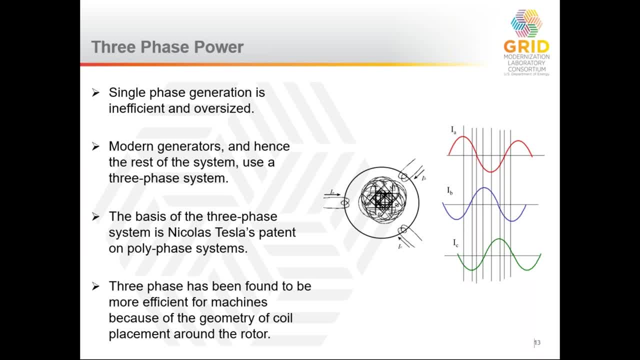 when we're dealing with tens, hundreds of megawatts, you'll have a three-phase system. As I said, the geometry of this makes it much more efficient. It was based on Nikola Tesla's patent of polyphase systems. Mathematically he extended it to more than three phases. 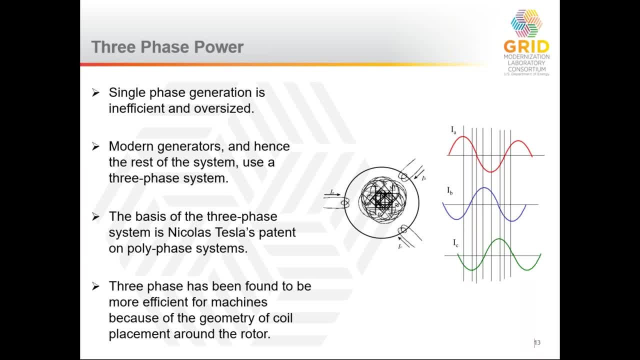 But what we find is that three phases really become a lot more efficient. Next slide should advance some animation. When you overlay these three phases- which is why we have three different conductors- you get this type of waveform here. It shows the three phases overlap with one another. 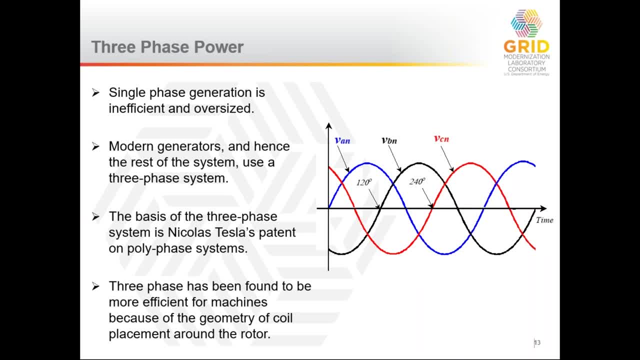 but this would be on three different conductors, And that's why, when you're driving down the road, you typically see three different wires on the overhead. Each of these will have one of the three phases- phase A, B and C- And so the generators will connect to all three phases. 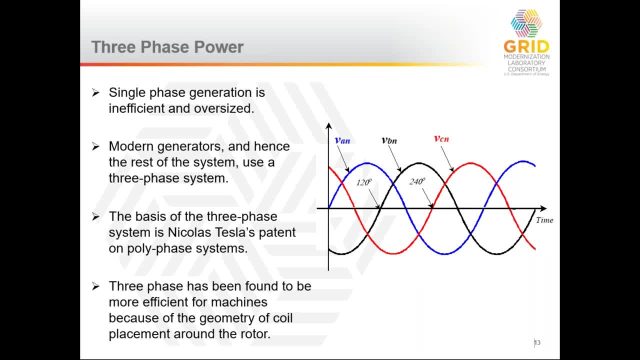 Large loads can connect to three phases, And so the generators will connect to all three phases, But typically customers, residential type, will only connect to one, And so this gives us the voltage source, and that will cause current to flow. Next slide, please. 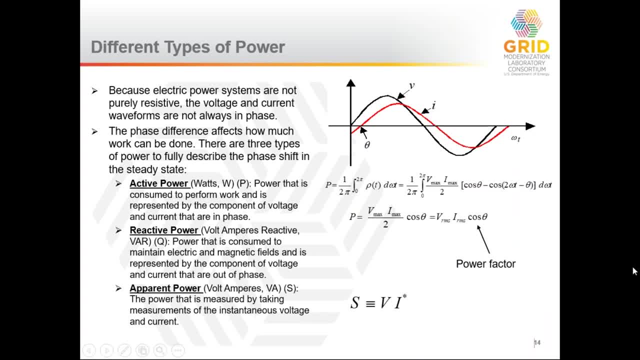 When you start talking about the voltages and currents. the next question is the different types of power, And this is a common thing that you'll hear folks in the utility realm talk about is that there's not just one form of power, And what I mean by that is. 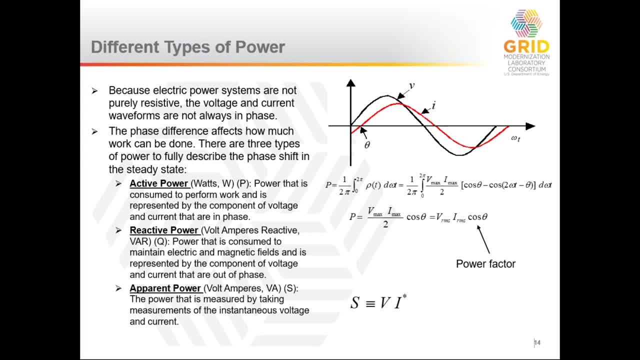 when you have a voltage that's moving in a sinusoidal form, the current will flow, but it may not flow exactly what's called the in-phase with the voltage, And what I mean by that is. we can see on this figure right here where the current and voltage 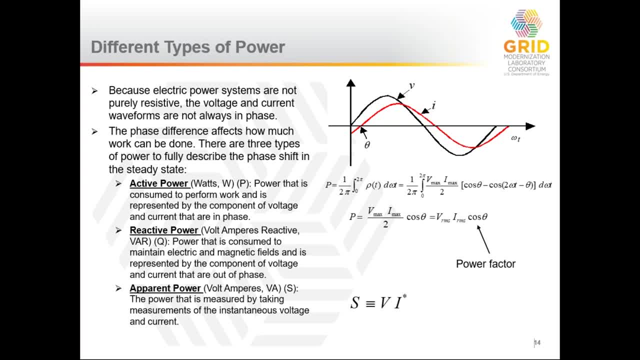 are out of phase. You can see that when the voltage is at zero, current is still flowing in the system And, conversely, there's times when there's no current flowing but there's voltage applies. This is caused, called a phase shift, And various elements in a power system can cause that. 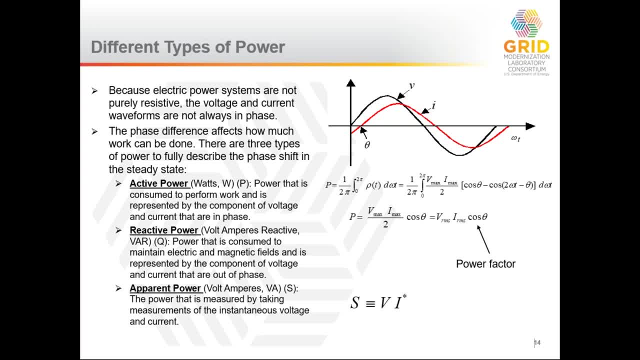 If everything is just resistive, like space heaters, this will be in phase. But because we have other elements in the system, such as inductors and capacitors, we'll get this phase shift where current will either lead or lag the voltage, And this results in different types of power. So first is the active power. 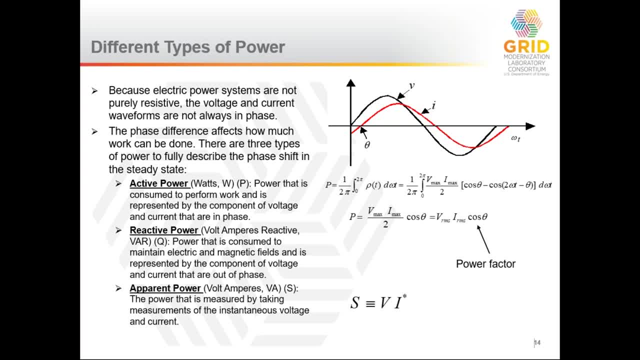 and the physics definition of this is power is going to be consumed to do work, or consumed to work in the physical sense, And so this could be heating something up, moving an object. This is actually what is useful to us, And it's the component of power. 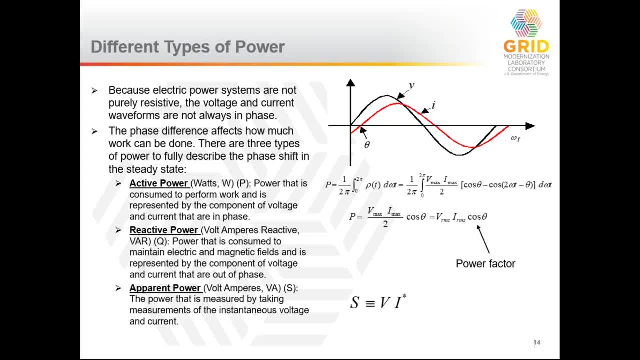 sorry- voltage and current that are in phase with one another. The reactive power: this is the power that is consumed to maintain, I should say establish and collapse electric and magnetic fields in the system, on your inductors and capacitors, And it is represented by the 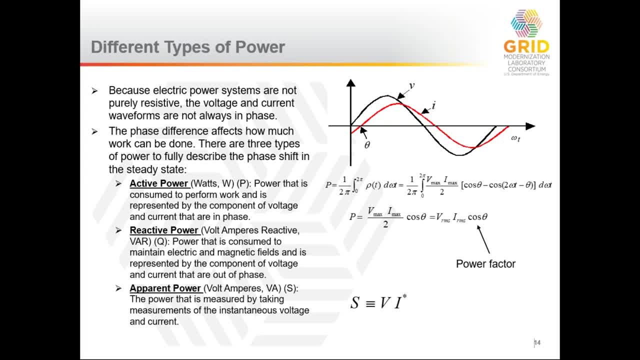 component of the voltage and current that are out of phase with one another. And then, finally, apparent power. this is the power that is consumed to maintain. that's measured by taking instantaneous measurements of your conductors. If you look at, if I measure the magnitude of voltage and measure the current Next slide, please, These three can. 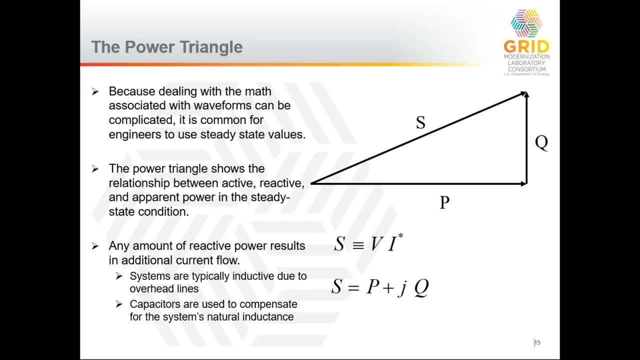 be related to one another, and these become very important concepts when you're looking at how you rate the various pieces of electrical equipment. While the active power, P, may be what we really want, we know that there is some amount of Q, the reactive power, that also ends up flowing. 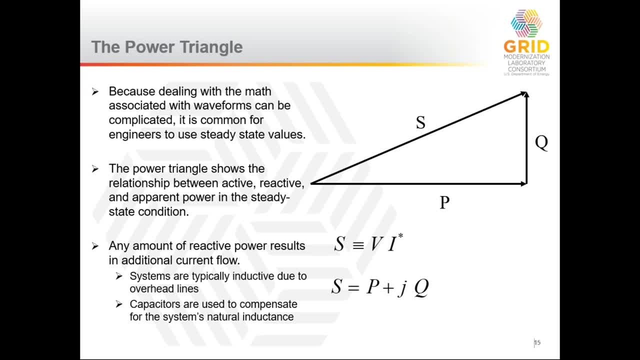 through the conductors, And so what you see is that the apparent power S- it's the hypotenuse- of P and Q. P and Q are at right angles to one another, And so where this matters is the amount of current that actually has to flow down the conductors. It's based on S, which is the 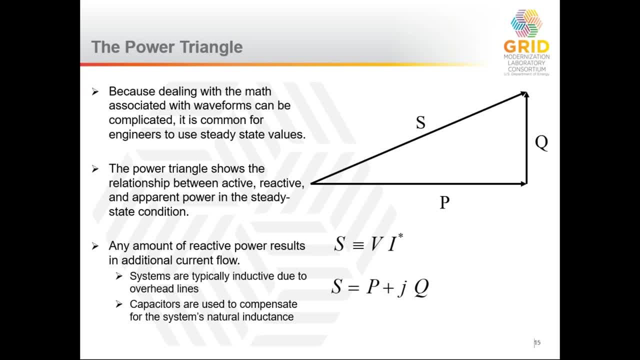 apparent power. So what we see here is that, while we may only want the active power P, we have to supply some reactive power, And in the process of that, that draws more current down the lines which heat things up. And so the result is: either you need to have larger, more 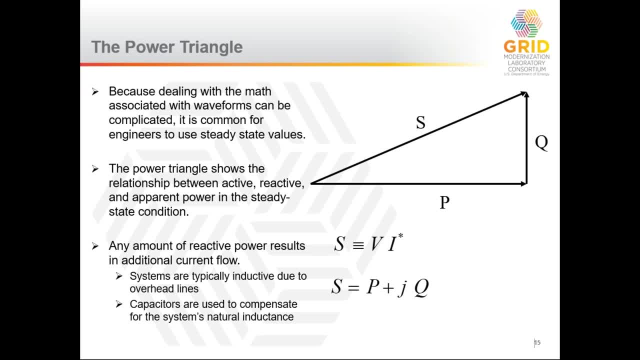 efficient equipment or you have to look at how that's going to impact the lifetime of that equipment. So it becomes a bit of a trade-off. When you talk about the different equipment and electric power systems, they have multiple ratings. Typically things like: 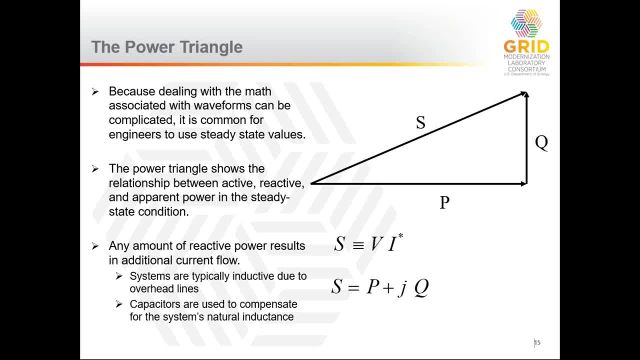 transformers will be represented in apparent power S, either KVA or MVA, being kila or million, And because really what you're looking at is the thermal ability for that to carry. However, the distribution engineers will be going in and looking at how much active. 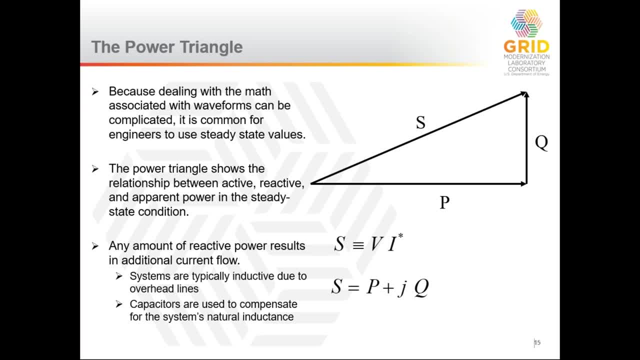 power do I have to provide to the customers, what elements are going to be consuming reactive power and how do I manage that? And that becomes a really big part of distribution system operations- is managing these three different types of power and their impact on voltage. 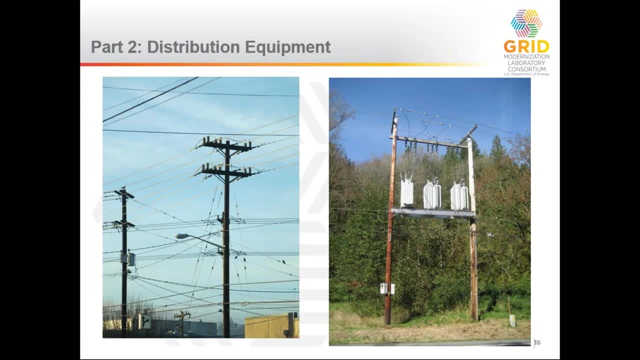 Next slide, please. And that brings us to the second part, where we're going to go in and start looking at some of the key pieces of equipment in electric distribution systems. Next slide, please. The most important part of a distribution system starts with the distribution. 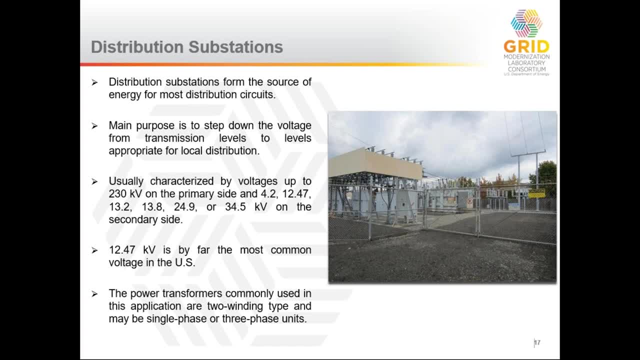 substation. For most distribution circuits, this is going to be the source of power that steps down power from either the transmission or sub-transmission system, So something on the order of 100 to 200,000 volts, possibly up to 230 or 500. And it will step it down with a substation. transformer to voltages that are typically low voltage, So that's going to be the source of power. Next slide, please. The most important part of a distribution system starts with the distribution substation. For most distribution circuits, this is going to be the source of power that steps down. 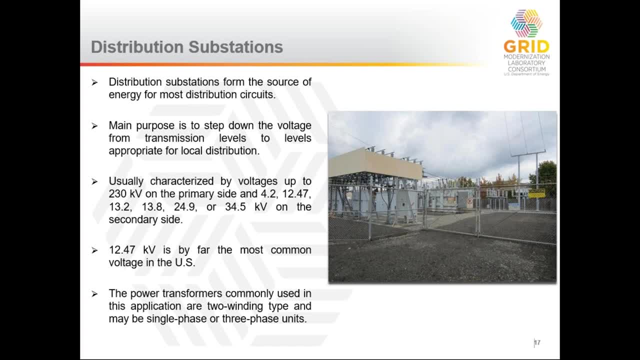 less than 50,000 volts. The most common voltage in North America is 12.7, sorry, 12.47 kV, But there are a number of other voltages used: 13.2,, 13.8,, 24.9, 34.5.. The trade-off is that 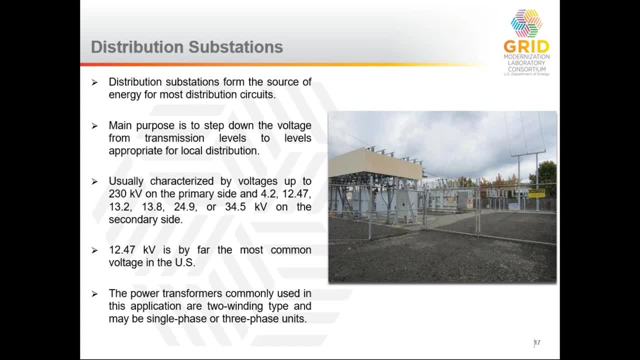 the higher the voltage. it allows you to move power more efficiently over distance. However, it requires larger, more expensive equipment, And so this is really the big trade-off that you see in picking these voltages. Now the challenge is that, once you, 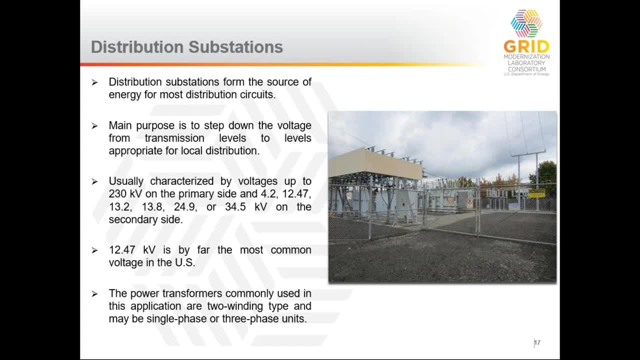 pick the voltage. all of the distribution system equipment uses that, And so if you decide to change the voltage over time, that requires changing out all of the equipment. That can be a very expensive and time-consuming process. I live in Seattle, which historically had a legacy 4.2 kV system. 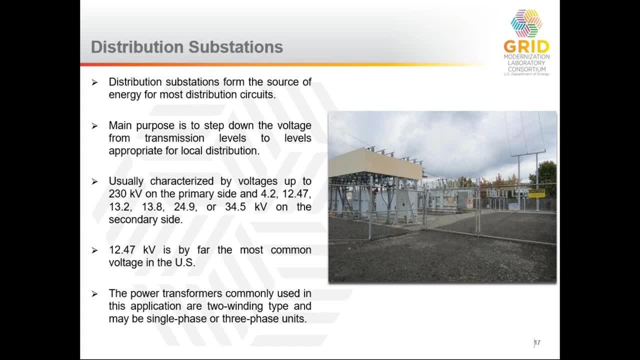 very low voltage, which required a lot of substations, But many years ago they switched to a 26 kV system. That changeover has been taking well over 20 years because of the life cycle of equipment, And so if you decide to change the voltage over time, that requires changing out all of the 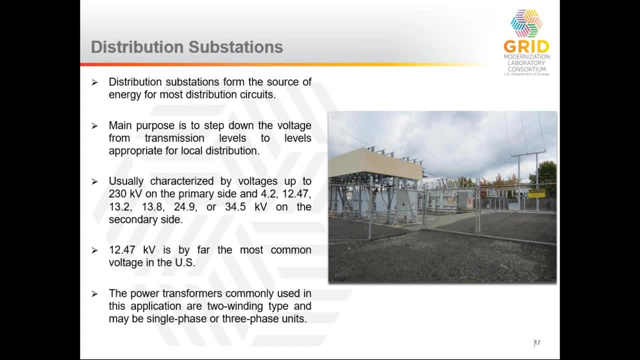 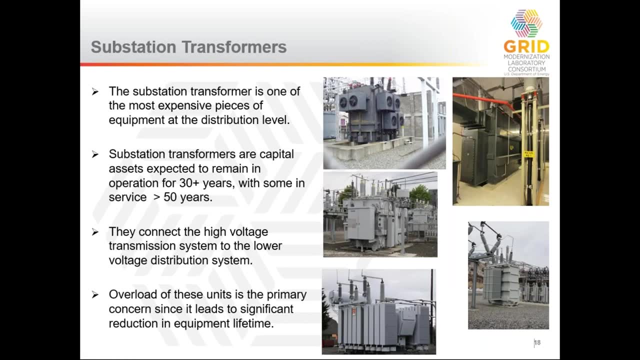 So the voltage is a very important aspect of this Next slide. please, Within the transformer. the single most important piece of equipment are the step-down transformers. These are large pieces of equipment that are designed to operate for 30-plus years. I've seen 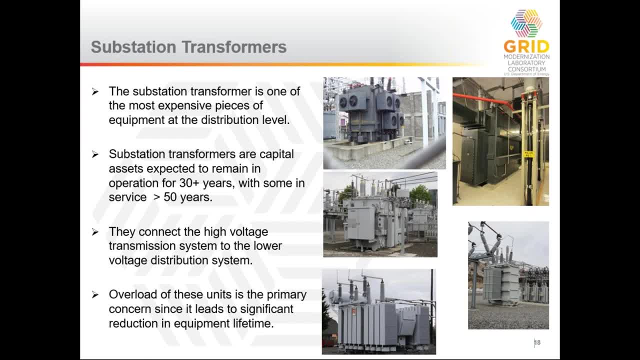 units in operation for over 50 years. Their primary function is to take the incoming power from the sub-transmission or transmission system, step it down to the lower voltage and supply that out to the distribution system, And so this is a very important aspect of this, And so if you decide to, 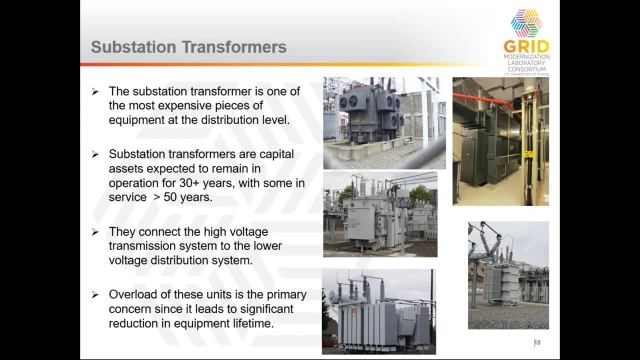 change the voltage over time. you have to take the incoming power from the sub-transmission or transmission circuits that head out into the system. The number one threat to these devices is heat. As you load them higher or put large spikes of power through them, that heating will degrade the internal electrical 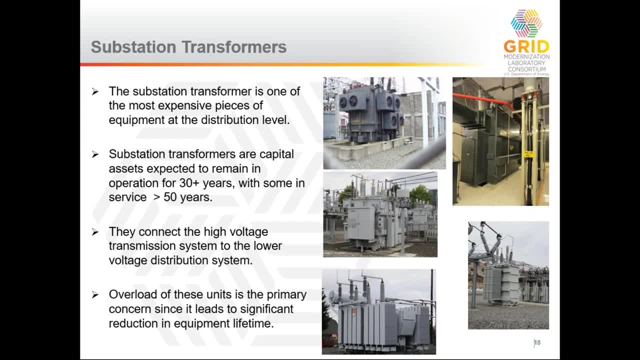 windings inside and that will reduce their lifetime, And so a lot of the operations around power systems are maintaining voltage, but also looking at what is the loading on the transformers and making sure they stay within their normal operating realm, You can see that these are actually pretty active devices in that the coils themselves are static. 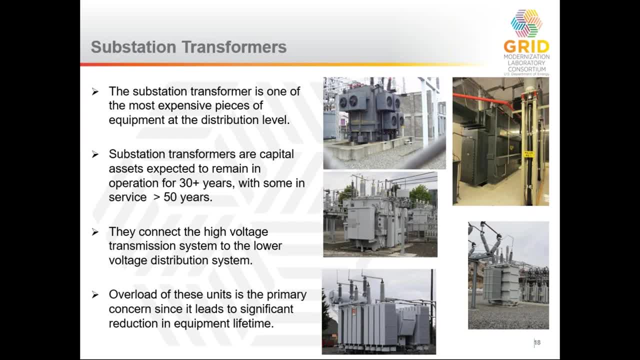 but some of these, such as the upper right hand, it's an interior building transformer. The exterior ones can have anything from passive cooling to forced fans to spray cooling. There's a lot of different ancillary systems that are designed to help these operate. 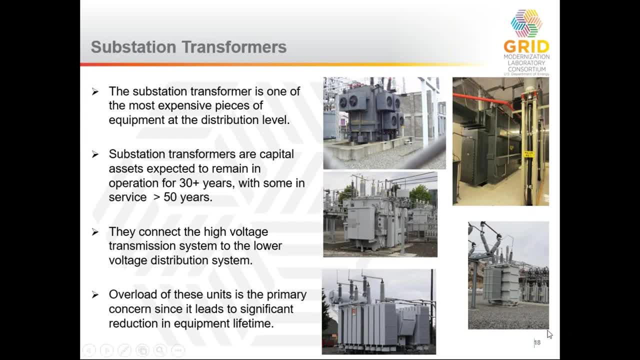 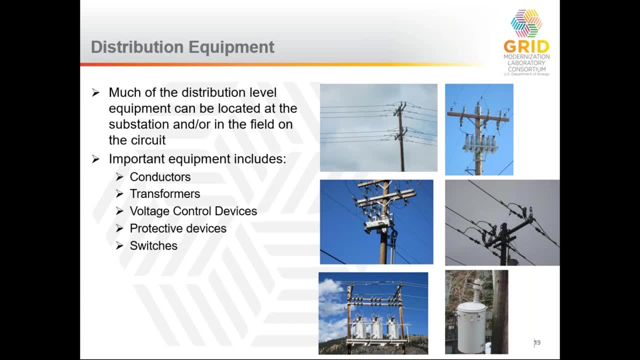 Next slide, please. Once you leave the substation, there's a large amount of equipment out in the field And really this is the vast majority of the distribution level equipment. This includes everything from the overhead conductors, which in the upper left hand. 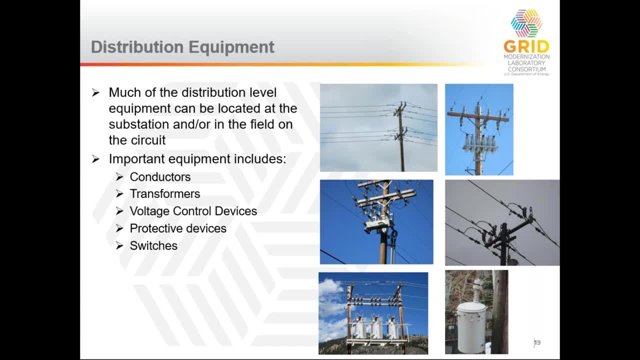 we can see an example of two three-phase circuits overbuilt one on top of the other. They will have a fourth common neutral down below them. It's just not shown in there. These are the overhead versions of it, But you'll also have transformers, typically the customer. 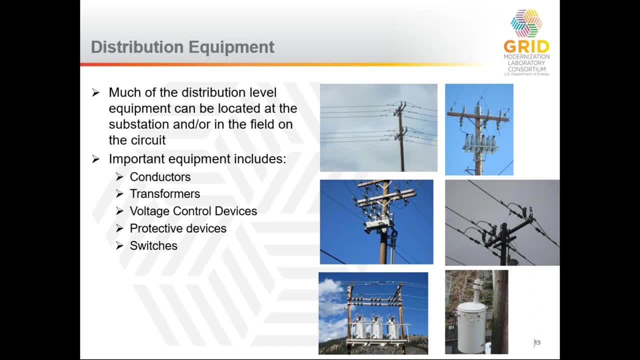 service transformer. an example of that shown in the lower right. The goal is to step it down to the 120-240 voltage that we use, But there are other pieces of equipment, such as voltage control devices, regulators, capacitors and protection systems. 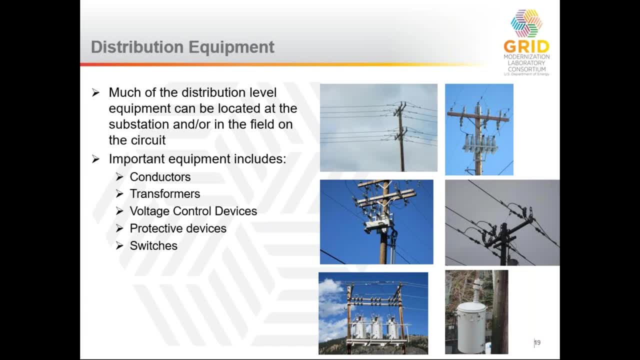 These are all needed to maintain the normal operating parameters of the distribution system and to protect it from credible events such as lines or trees landing on lines, animals, cars that strike the poles and drop them, and things of that type. And so there's a large amount of equipment out there, and replacing it once again takes a long time, because this equipment is designed to stay in place for a very long time. 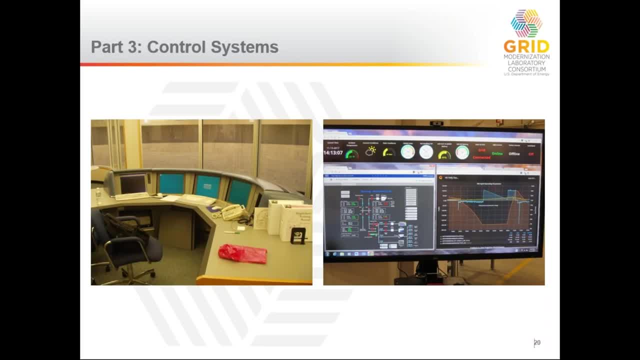 Next slide, please. Next part is to talk a little bit about how are all of these control? what are some of the basic control systems that can be used to operate this equipment? While much of this equipment exists out in the field, we're seeing a lot of modernization across utilities to start to look at how you can control it more efficiently. 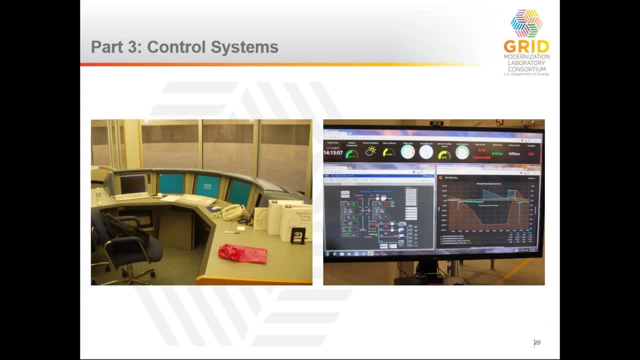 Historically, distribution systems were operated where you would build them out for maximum peak load and then they would passively operate on their own. This was efficient as long as systems were overbuilt, people weren't worried about too much equipment being put in the field and we didn't have a lot of active generation sources out there. 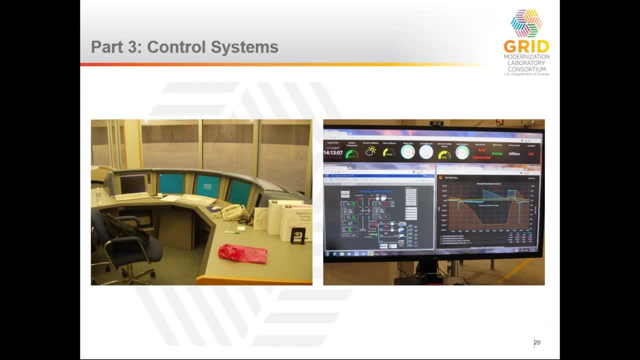 As that's changing, utilities are adapting to look at different control mechanisms for how you would maintain normal operations. What we have here on the left-hand side is a picture of a distribution control center, a very traditional looking setup, and on the right-hand side is a picture of a more modern microgrid control setup. 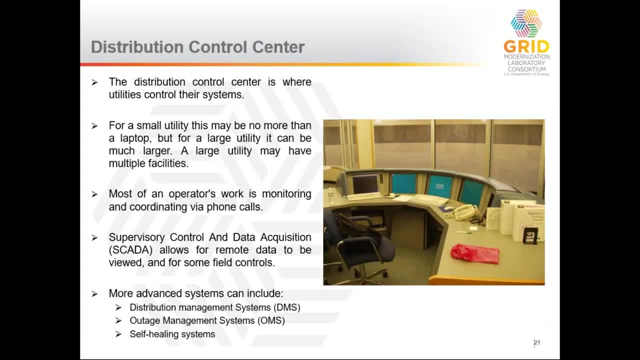 Next slide, please. The distribution control center. this is where utilities control their systems from. This doesn't look like the big movie boards where you have a perfect interface. This is a map of everything going on. There's 100% accurate situational awareness. 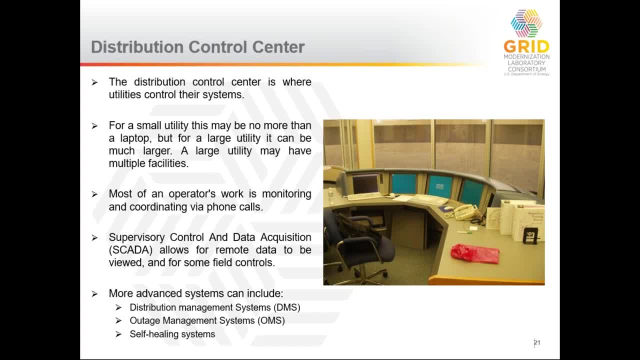 For a small utility, this may be nothing more than a laptop sitting in a closet. As you go to the larger utilities, they will in fact have big one-line MIMIC boards on the wall, many of them electronic. that will give them some operational visibility into what's going on. 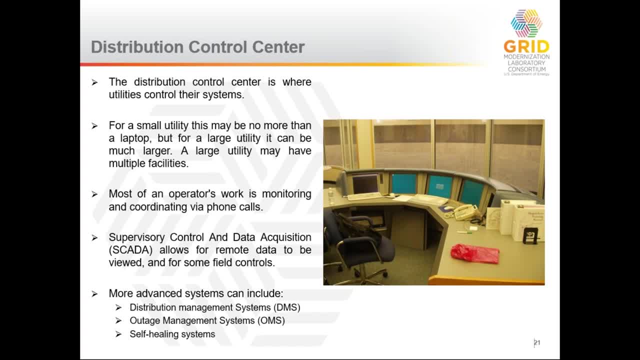 And so they can see what the current status of the system is. However, the level of automation is somewhat limited And most of an operator's work- Most of the operator's work- is really monitoring phone calls and coordinating operations with the field crews. 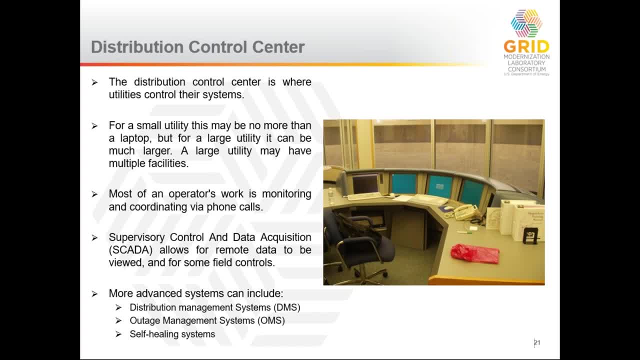 There are some operations that they can take, especially with self-healing systems and some of the automation, but the vast majority of their work is what's called switch management work. Now there are some remote pieces of information available. These typically use a supervisory, control and data acquisition or SCADA system. 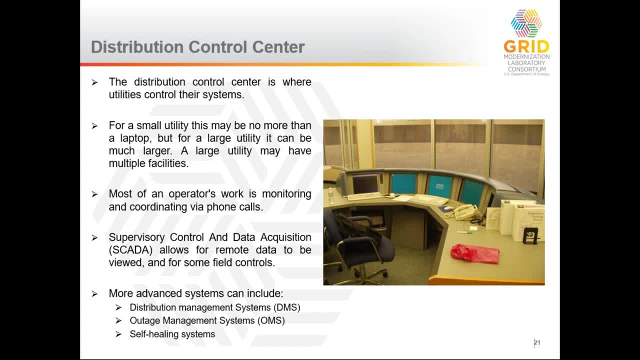 These systems have been around for decades and they're commonly used in power systems as well as oil and natural gas, But they are specifically designed to be able to read information from remote points in the field, dispatch control signals, and they are kind of the basic communication and control systems that utilities can use. 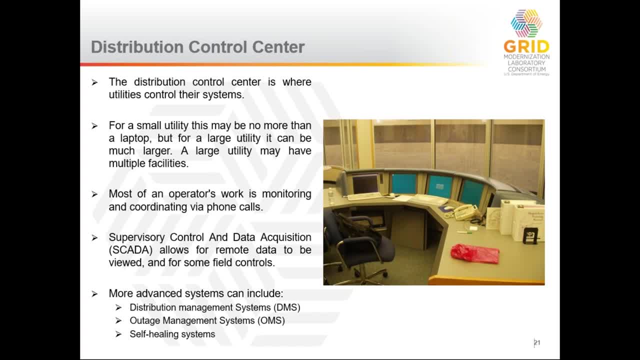 These in themselves do not have a lot of advanced functionality and they are brought together with more advanced systems such as distribution management systems, outage management systems, self-healing systems, and they can work together to implement these systems. The resulting supply chain is basically amazing: you can go from the remote to the touch on the receiving end. 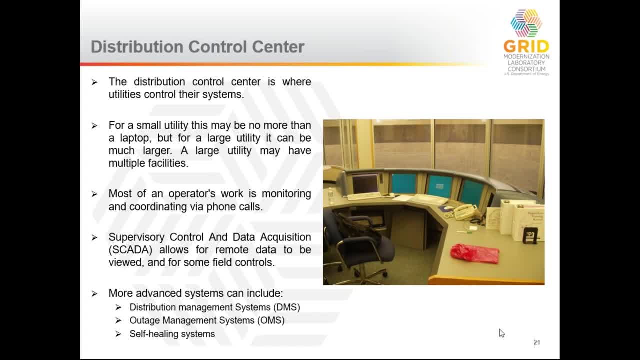 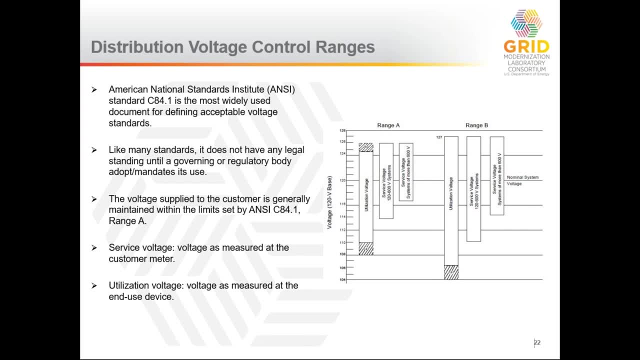 And you can also use the remote permission from the Mexico phone and call them to take advantage of insurance Xinore's embedded system like trainingket. Next slide, please. One of the basic functions that is examined is voltage control. Voltage control is probably the single most important operational aspect after making sure the system isn't overloaded. 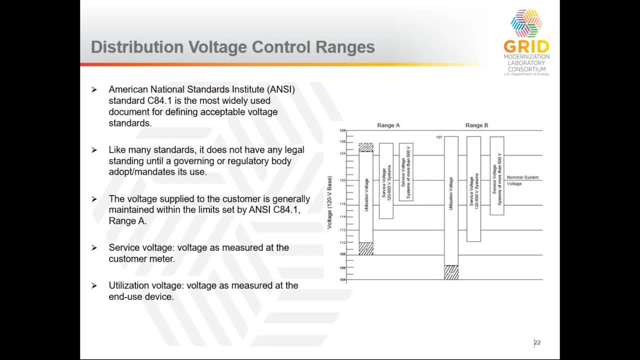 That utilities have to worry about. In North America, the most commonly used the standard is the ANSI C84.1.. Most public utility regulators have access to this standard. You should follow the filtered data from the Americanлавage page here. You should follow the filtered data from the Americanlave page here. 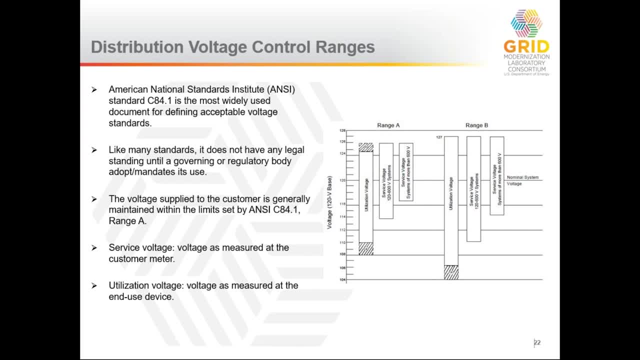 The DCR installed Most of the human resources related to up cooling and heating equipment this year, already have access to regulators. they will go through and select this as the standard and what it does is basically say here's the range they should remain within, and it's typically 120 volts, up to 126 and down to 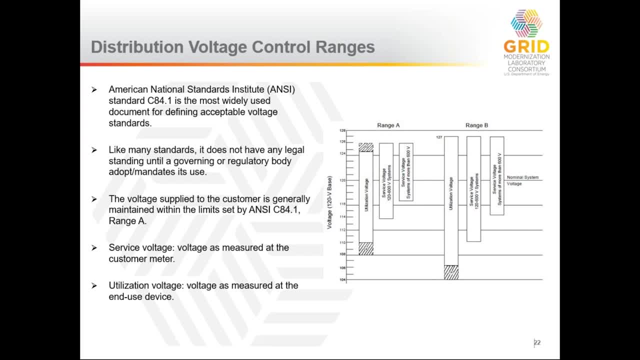 114,, so plus or minus 5 percent. This standard on its own does not have any legal standing until a regulatory body sets it as the standard. and this is the voltage as measured at the customer meter. Now I mentioned on the 120 volt scale, but really single-phase residential houses receive 120,, 240,. 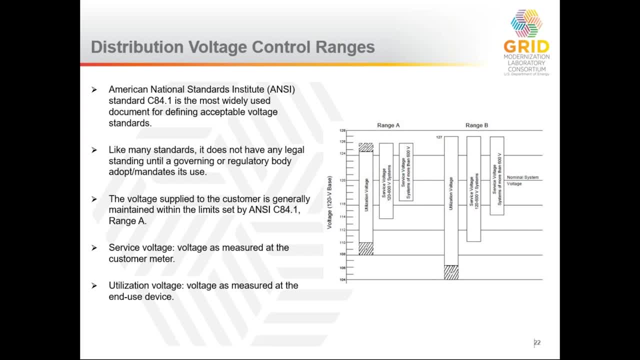 so this can be scaled to the 240 as well. There is also another range B which can be used under other ranges if there's an abnormal situation. This is once again up to the discretion of the Utility Commission. Next slide, please, When you look at an operational distribution system. 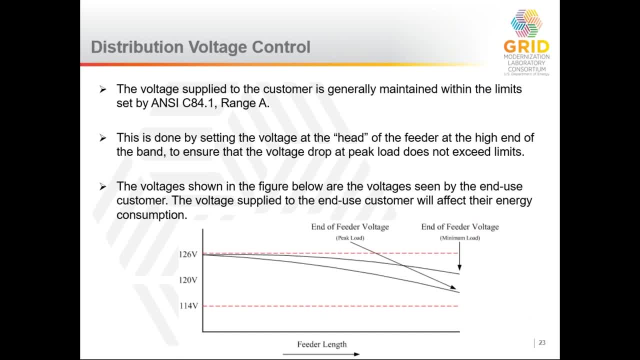 it is almost always maintained within the range A limits of ANSI. The traditional way this is done is you take the voltage at the head of the distribution feeder or circuit, which is the substation, and they set it at the high end of the ANSI band, typically around 125 volts, and then 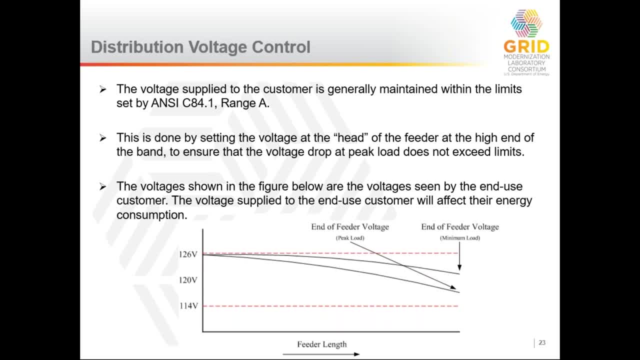 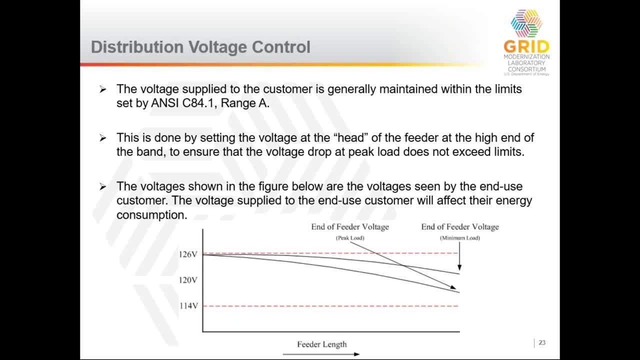 but it will vary how much it drops over the course of the day. And in this figure you can see two different traces where you have the end of feeder voltage at minimum load and peak load. At peak load, the highest load of the day, you see the voltage brought down a lot more than it is during. 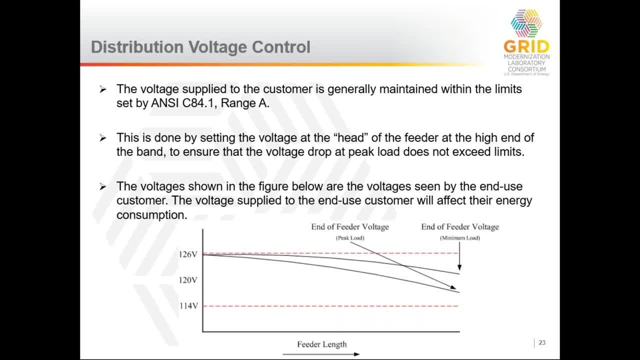 the peak load, And this is also keep in mind. this is a conceptual drawing of an idealized single line going out. In reality, distribution circuits sneak out in many different directions So it's not as easy as a simple profile like this, but for a conceptual understanding you can see how these are operated. 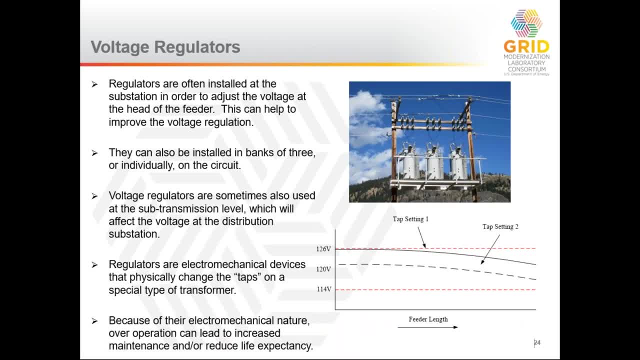 Next slide, please. For situations where the voltage can sometimes the voltage drop, can become too high, utilities will deploy what are called voltage regulators. These are smaller transformers that are designed to be able to regulate their output voltage within a range, And so these are electromechanical devices and they can be referred to as tapping up or tapping down. 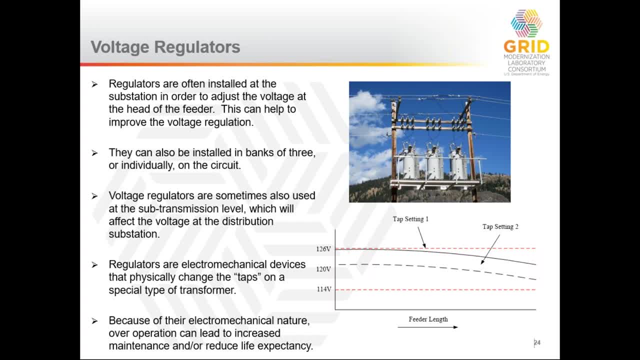 And what we see here is an example of two different tap settings, where the dotted line is a lower voltage tap setting, where it's set at just above 120 volts and the second one is set at 126 volts. And so you can see, in this case you can move the voltage of the head of the feeder up and down, which will affect the voltage down the entire system. 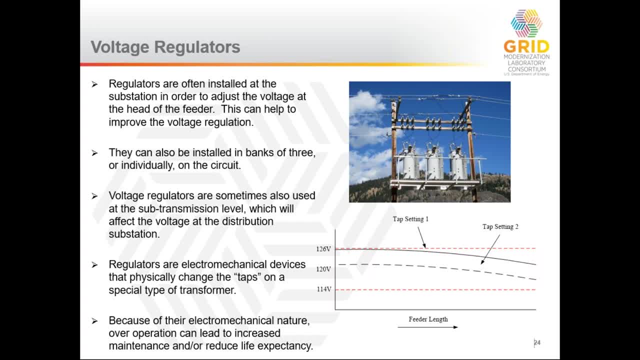 That level of flexibility allows you to accommodate For changes of. as the load changes in the day, you can go ahead and change your tap positions so that customers don't see the voltage drifting over the full range of the day. By actively tapping throughout the course of the day, you can keep the voltage in a much more narrow contained band. 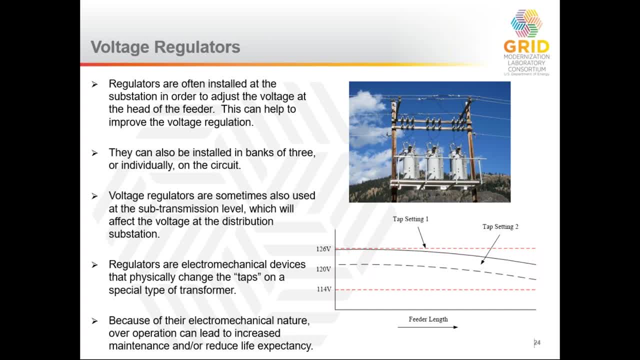 And for most utilities. you can even see this in your house. if you go put a meter to the outlet, it'll only vary a little bit. Now, this can depend on where you live. If you live in an urban area with a strong system, you may not see this. 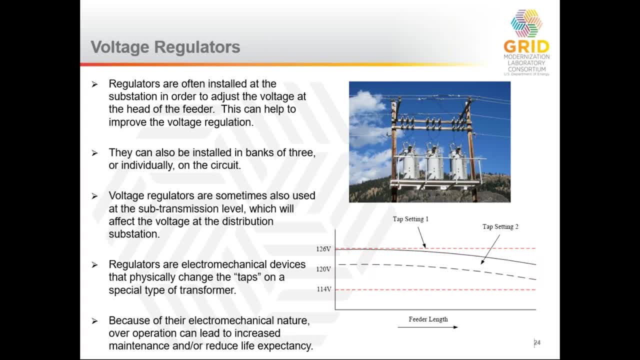 You may not see much voltage variation. If you're in a very rural community at the end of a circuit, it potentially could change quite a bit. Next slide, please. Here's another example of putting a regulator further out of the substation, because sometimes you can have a situation where, even if you move the voltage all the way at the head of the feeder, the top end, you still may violate the low end by the end of the circuit. 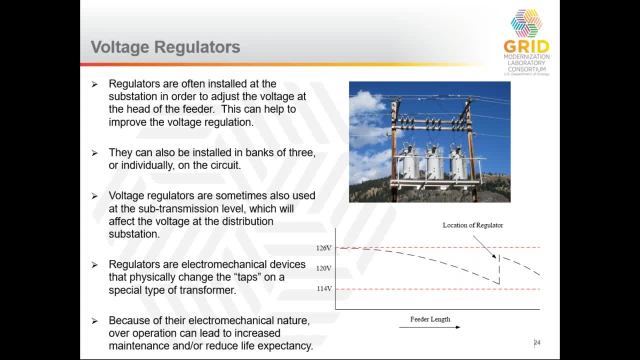 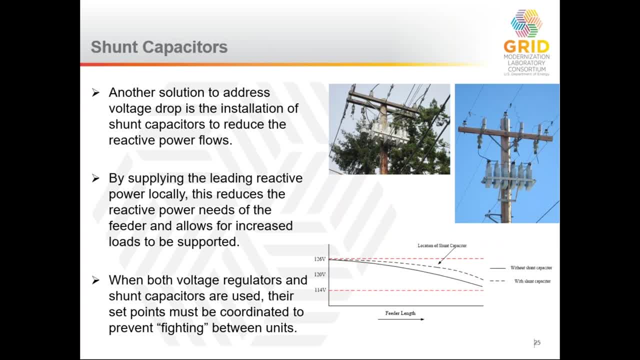 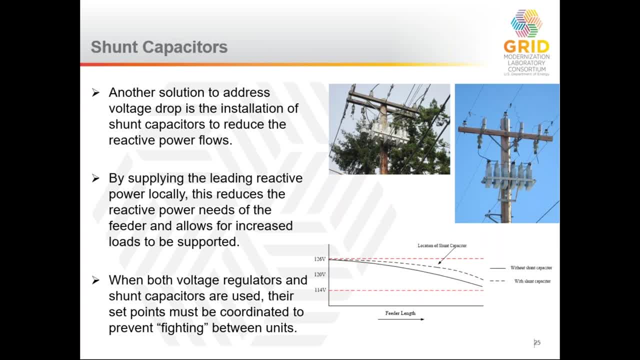 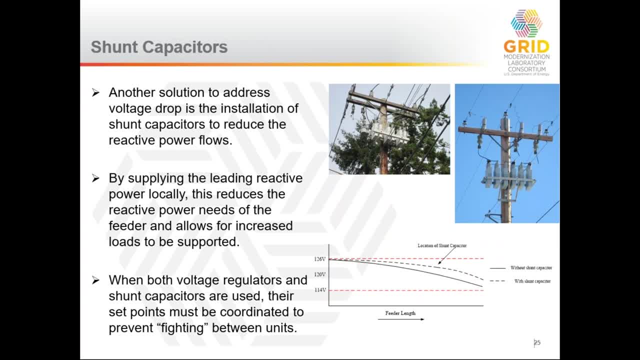 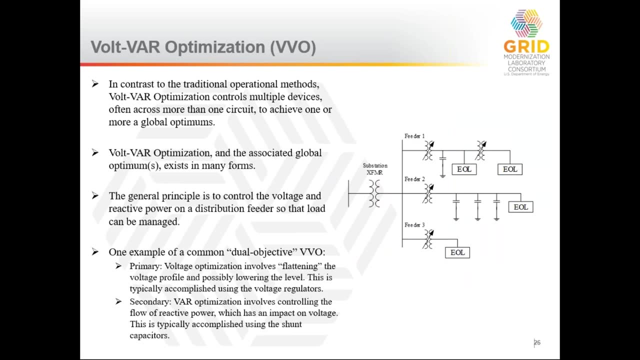 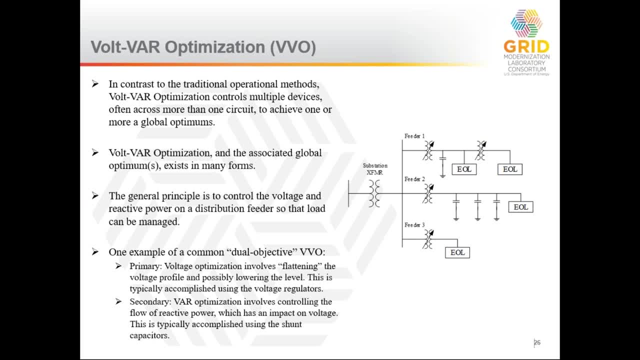 and this is done to optimize the system, and so what it does is it tends to flatten the voltage profile across the entire distribution circuit, pushes it down to the low end of the acceptable band, and this has the effect of reducing the overall energy consumption, and so it makes the system operate more efficiently. and it's been well shown that if you operate on the low end of that band, loads will still provide the same quality of service. they just operate more efficiently, and so this is an example of one of the 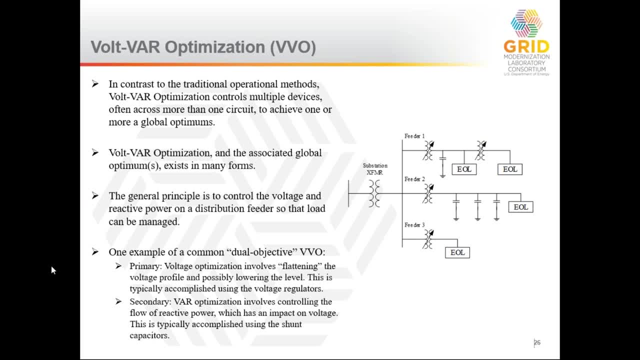 newer type of technologies. I should caveat: newer because VoltVar optimization in various forms, has been around for 30 plus years, although it's becoming much more advanced these days because we have better communication systems. the SCADA is much better, the control systems are a lot better and so is the computing power. so there's a lot of schemes out there for how can you optimize this information, and so I'm showing, on the right hand side, a very simple example of a substation transformer with three